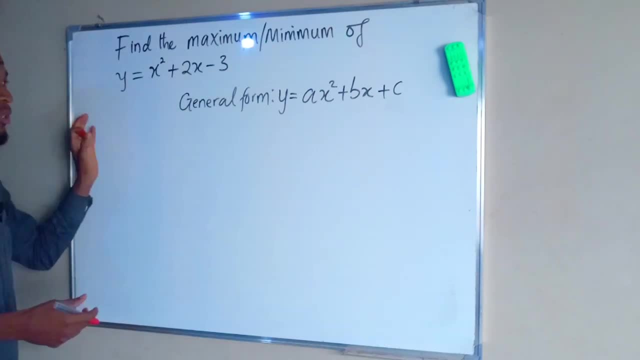 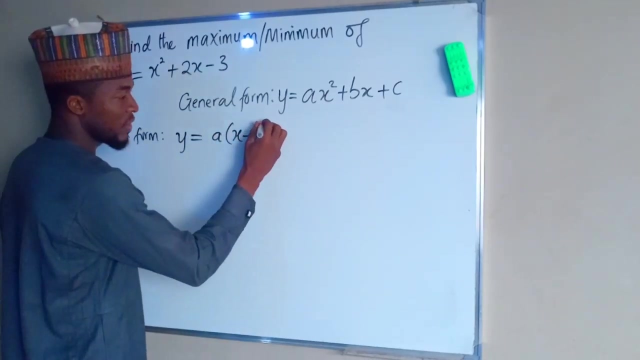 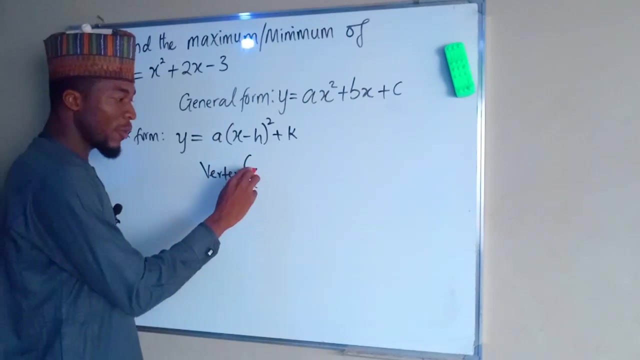 function function. so the very first method I'm going to use is by transforming the quadratic equation into vertex form. the vertex form of a quadratic equation is given as: y equals a, x minus h, squared plus k, vertex is a coordinate of h and k. so if you have a negative value here, 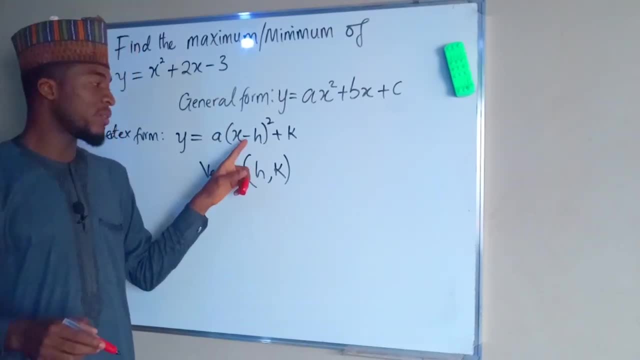 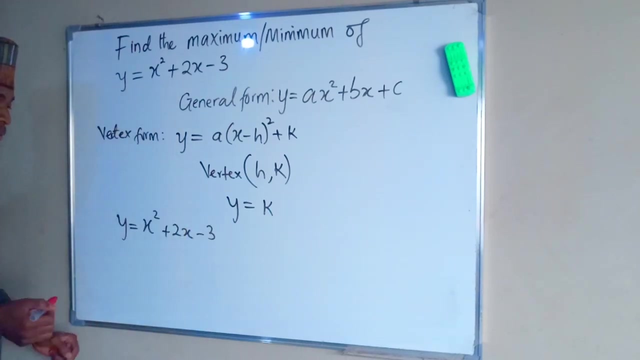 you are going to obtain the positive one. if it is positive, you take the negative. the minimum of the quadratic equation is going to be: y equals to k, this value, this particular value. so now let us see how we can transform this. the equation is given as first step. you are going to group the 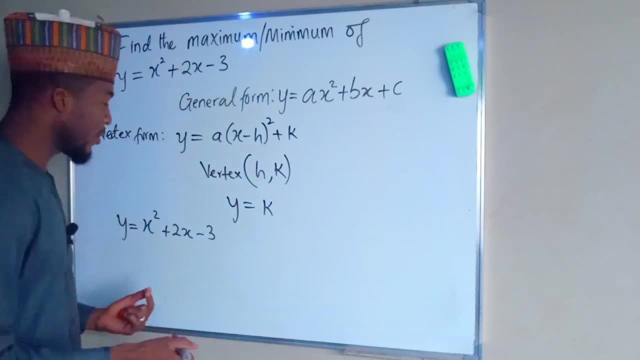 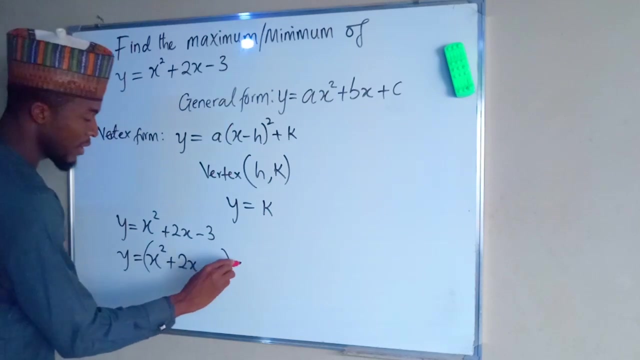 first and the second term and let the third term alone, which is the constant term. so we are going to have something like this: x squared plus two x. you give a space because we are going to add a particular number here, the minus 30, which is this term, the constant term. we are going to transform these two times into a perfect square. 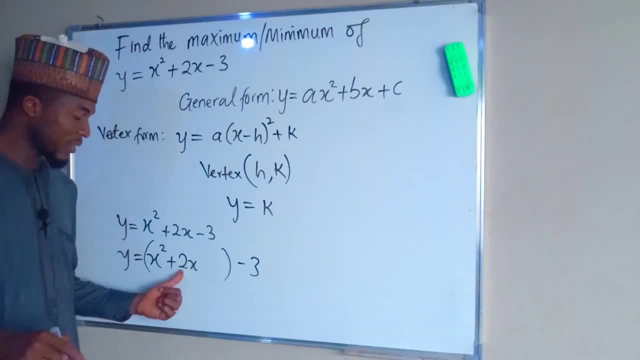 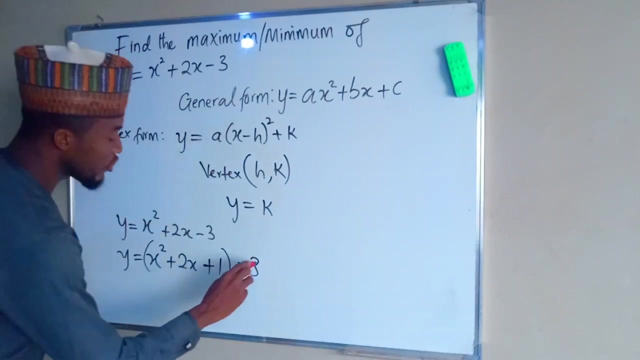 we're going to take half of the coefficient of x, which is one, and square it, and it's still going to give us one. then we add one here. this is a perfect square quadratic function. we have added one to the quadratic function, but initially it does not have one, so we are going to subtract to the other side. 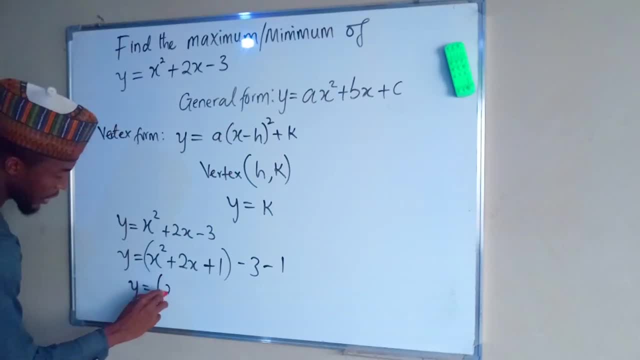 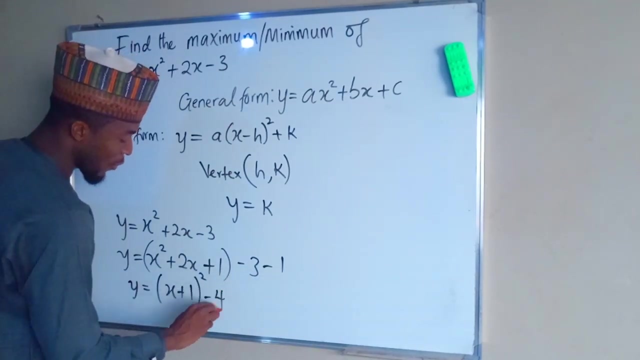 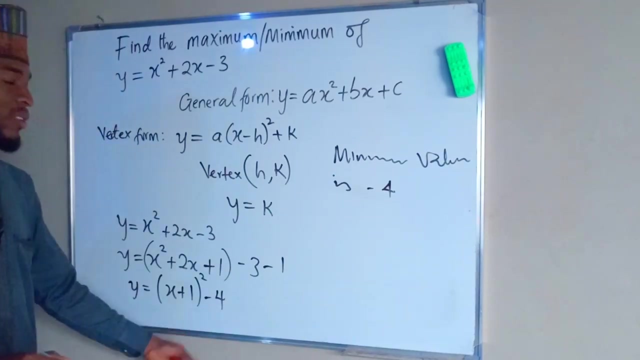 y now equals x, because it's the fifth square plus half of the coefficient of x, which is one squared. the minus three minus one is minus four. the minimum value is minus four and minus four, you know, is the value of y. this is method number one. then method number two: 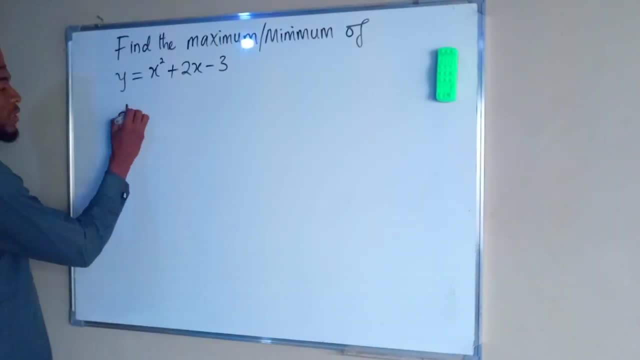 we are going to take the derivative of this function, dy over dx, which is also a slope. if you differentiate this first term, you're going to obtain 2x. if you differentiate the second time, you are going to obtain two. and the last time, which is a constant time, the derivative of a. 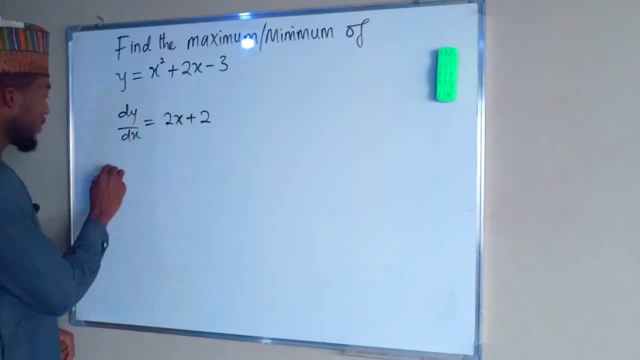 constant term is zero. we are going to solve for x at dy over dx equals to 0. So we are going to obtain: 2x plus 2 equals to 0. Then 2x will be equal to negative 2.. If you divide both sides by 2,. 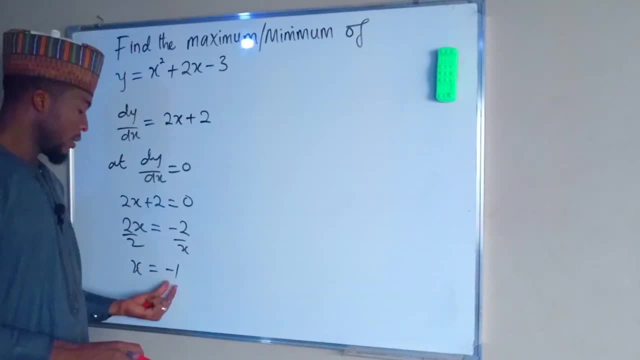 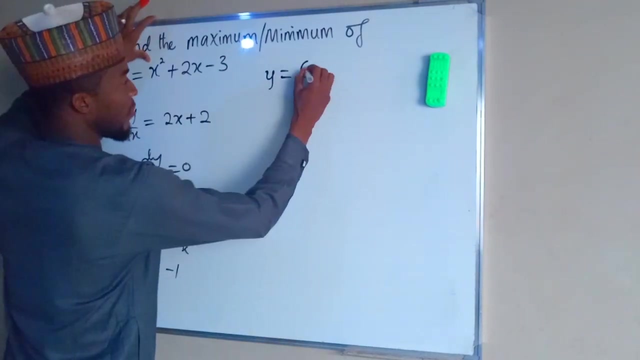 x will now be equal to negative 1.. This value of x equal to negative 1 is the value of x at the vertex of that quadratic graph. So we are going to substitute for x in the main equation y equals to. then we substitute for x minus 1, squared plus 2 times minus 1, then minus 3.. 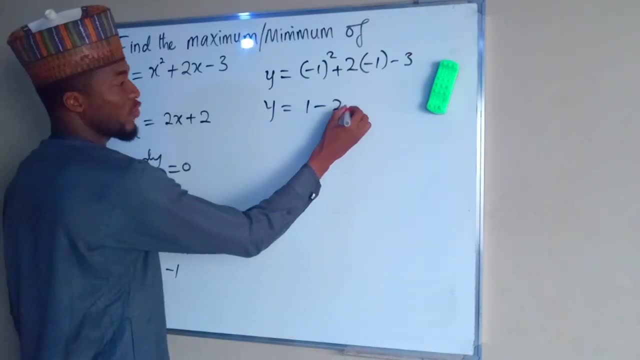 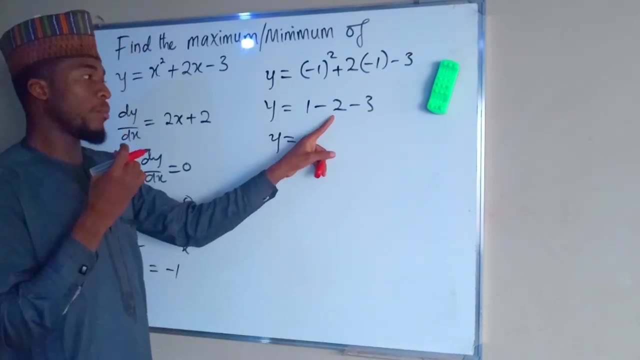 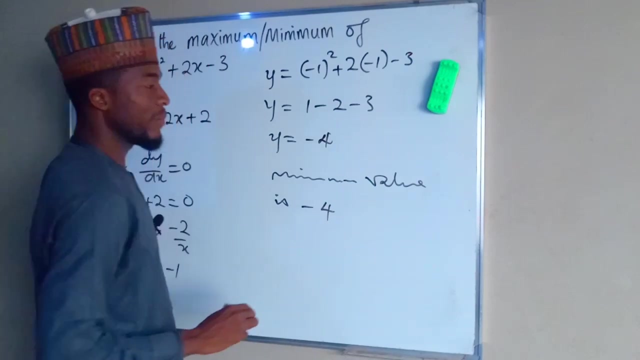 y will be equal to. this is 1, minus 2, minus 3.. y equals 1 minus 2 is minus 1, then minus 1 minus 3 is minus 3.. Therefore, the minimum is minus 4, the same answer. 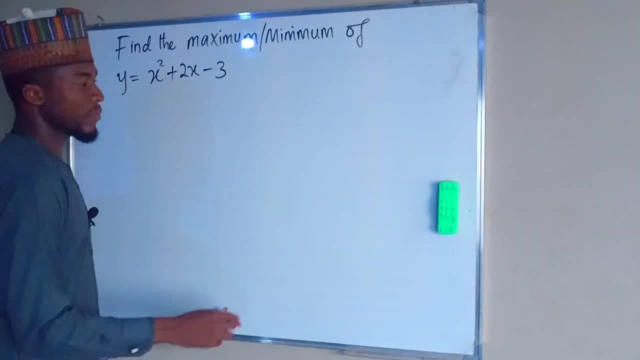 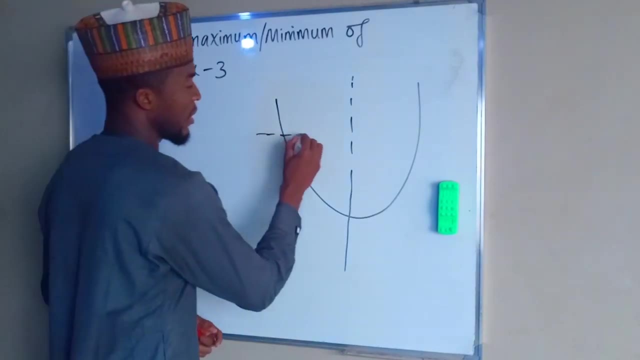 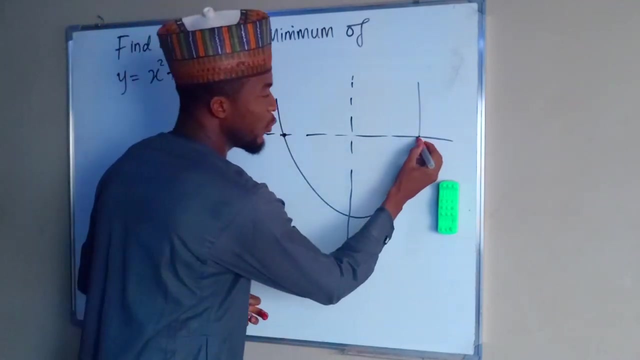 By using the value of x at line of symmetry. the line of symmetry is a line that divides a parabola into two equal half, and it's also a value of x. And to obtain that value, you are going to add the two roots of that quadratic equation and divide them by 2. You are going to obtain the value. 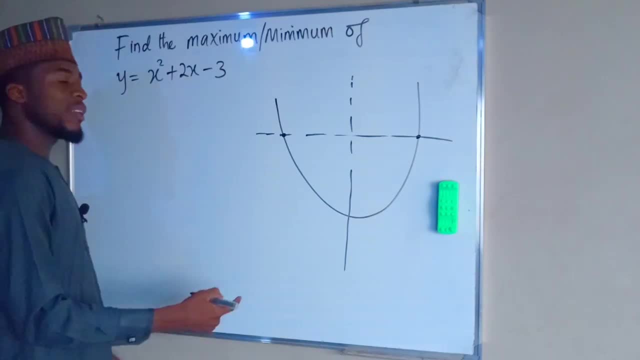 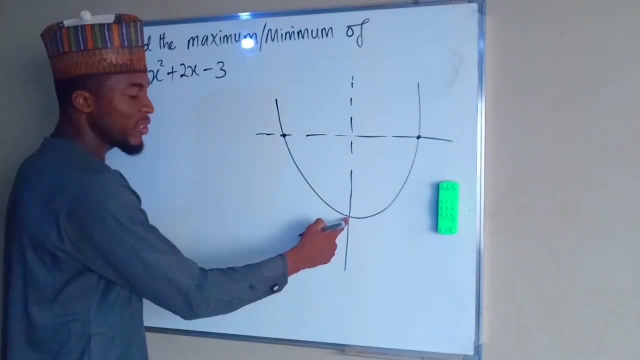 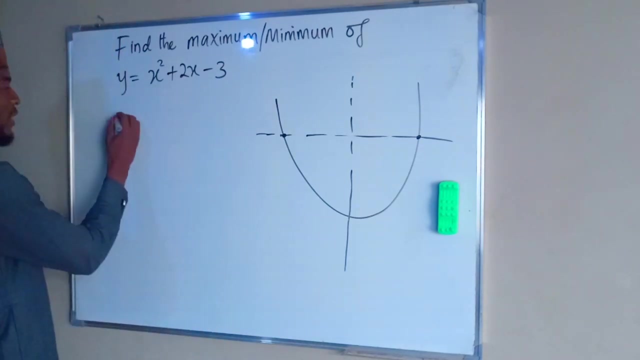 of x, Add the line of symmetry, and the line of symmetry will lead you directly on the peak, which is the vertex of that quadratic graph, and the corresponding value of y at that point is the minimum value of this quadratic equation. That is a shortcut for that one x equals to negative v divided by 2a. 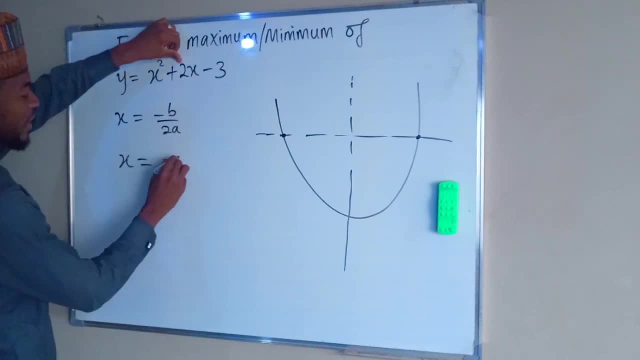 And now x equals to negative, b is negative, 2, divided by 2, times the coefficient of x squared, which is a, and it's 1 here, and this will give us minus 2 divided by 2, and now x. 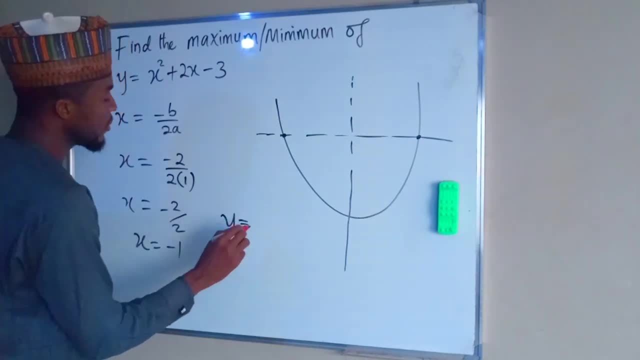 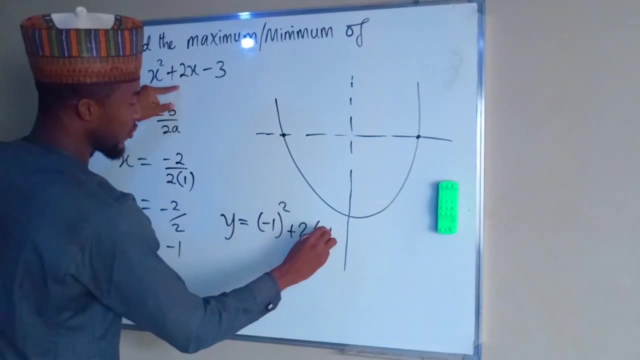 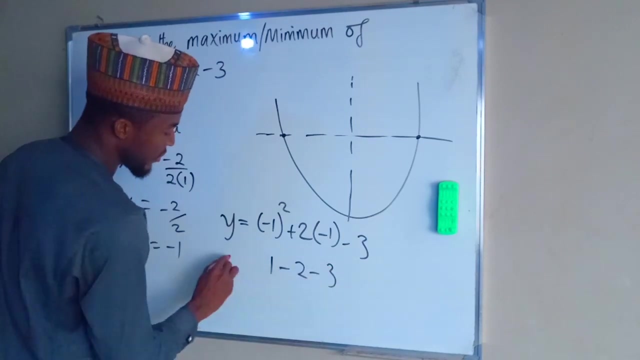 equals to negative 1.. Now y equals to minus 1, squared plus 2 times minus 1, then minus 3.. This is 1, minus 2, minus 3.. This is the value of y, and y equals to minus 4..